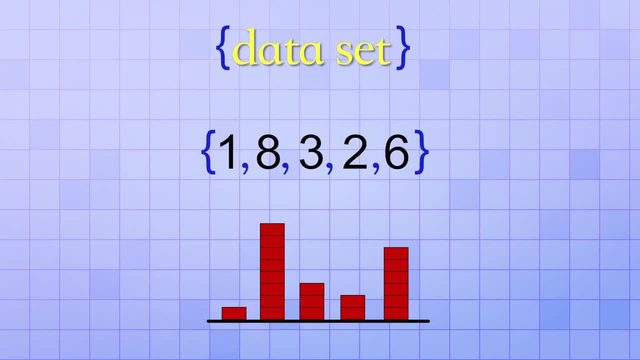 As a visual aid, let's also represent those numbers with stacks of blocks whose heights correspond to their values: 1, 8,, 3,, 2, 6.. Right now, since each of the five numbers is different, the stacks of blocks are all. 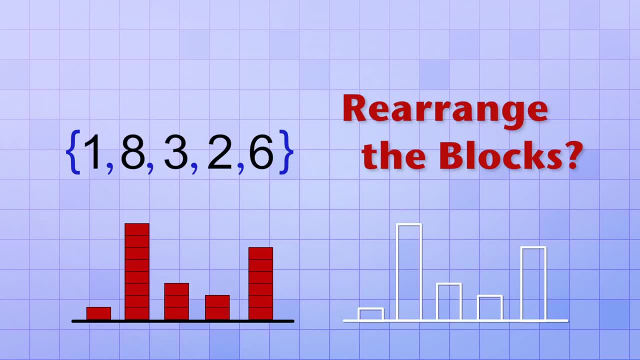 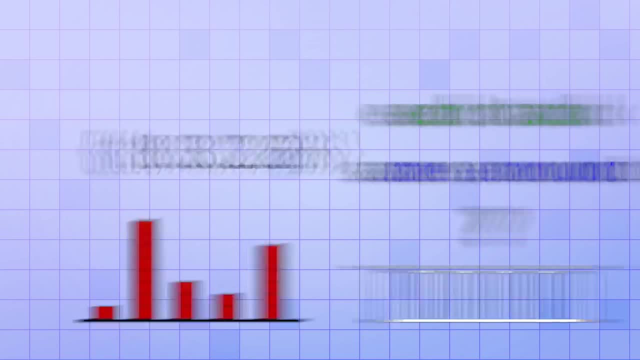 different heights. But what if we rearrange the blocks with the goal of making the stacks the same height? In other words, if each stack could have the exact same amount? what would that amount be? Well, with a bit of trial and error, you'll see that we have enough blocks for each stack. 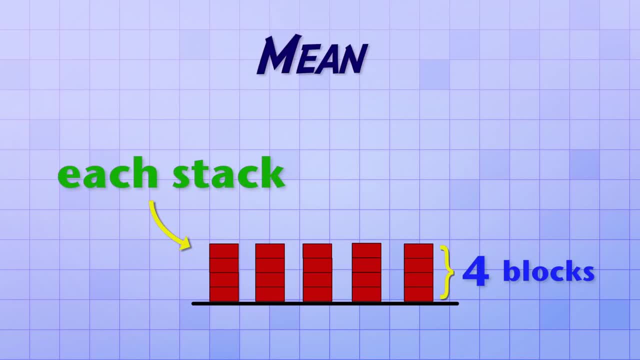 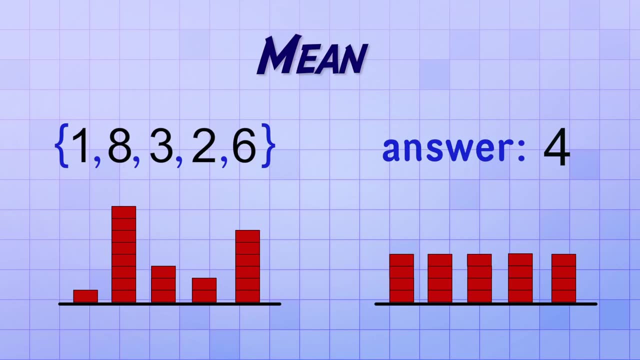 to have a total of 4.. That means that the mean or average for our original dataset would be 4.. Some of the numbers are greater than 4 and some are less, but if the amounts could all be made the same, they would all become 4.. 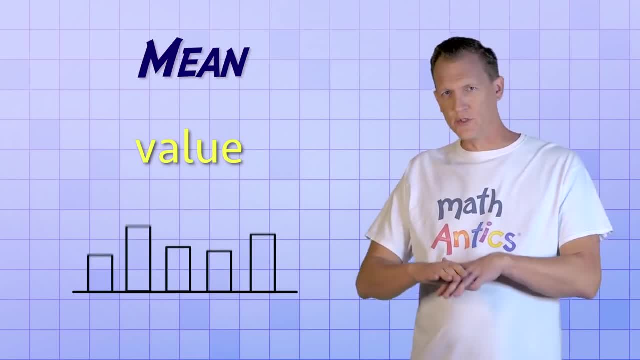 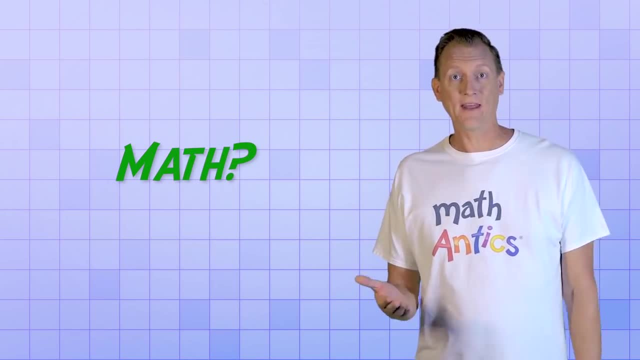 So that's the concept of the mean. It's the value you'd get if you could smooth out or flatten all of the different data values into one consistent value. But is there a way that we could use math to calculate the mean of a dataset? 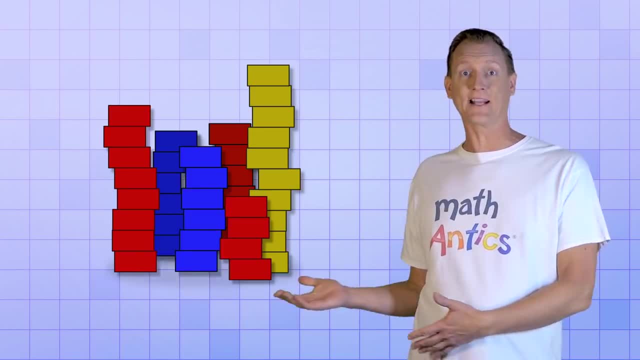 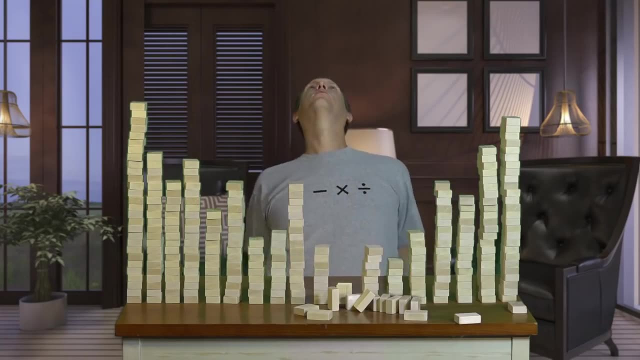 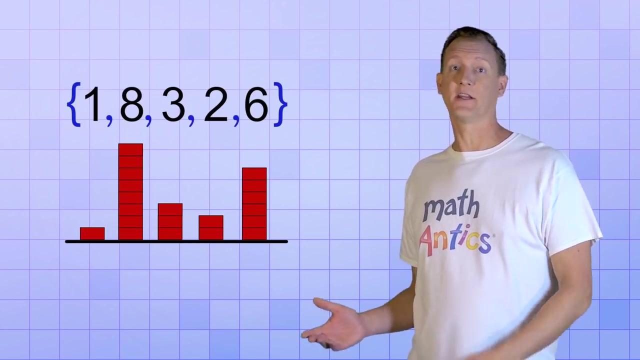 After all, it would be very inconvenient if we always had to use stacks of blocks to do it. There's gotta be an easier way. Oh man, Phew, It's easier for calculating the mean. let's start with blocks again, but this time instead. 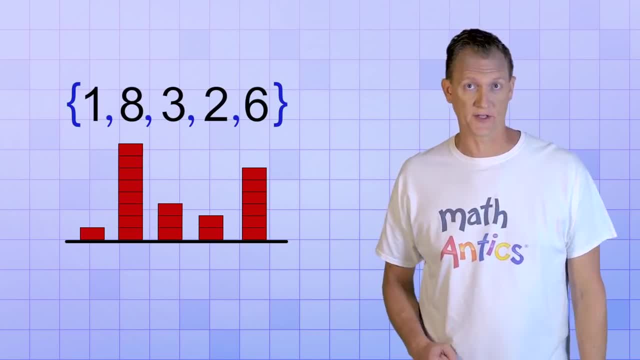 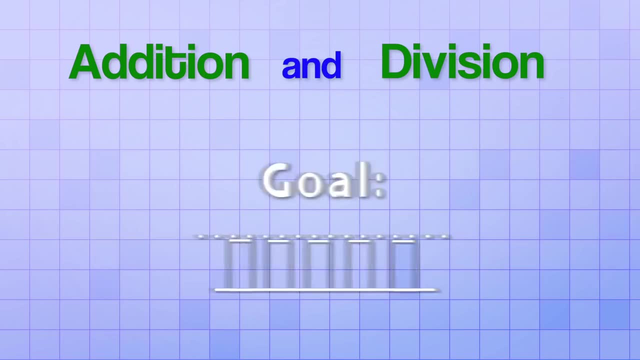 of using trial and error, let's use a more systematic way to make the stacks all the same height. This way involves a clever combination of addition and division. We know that we want to end up with 5 stacks that all have the same number of blocks, right? 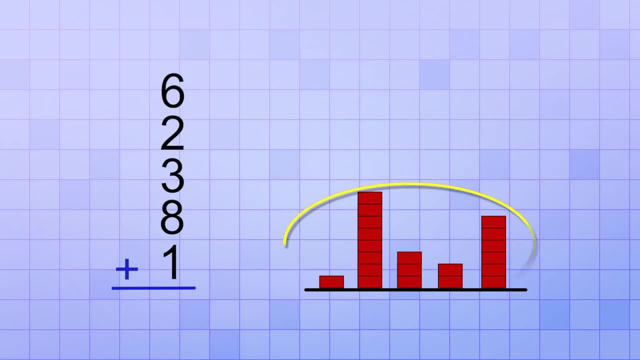 So first let's add up all of the numbers, which is like putting all of the blocks we have into one big stack. Adding up all of the numbers, or counting all the blocks, shows us that we have a total of 20.. 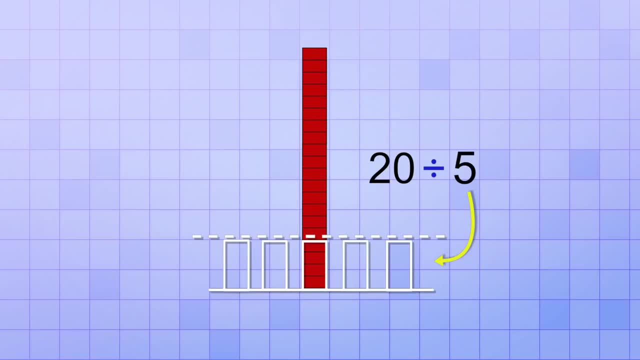 Next, Let's divide the total number, or stack, into 5 equal parts. Since the stack has a total of 20 blocks, dividing it into 5 equal stacks means that we'll have 4 in each, since 20 divided by 5 equals 4.. 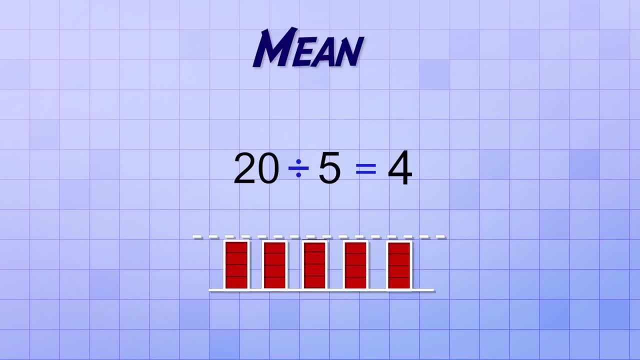 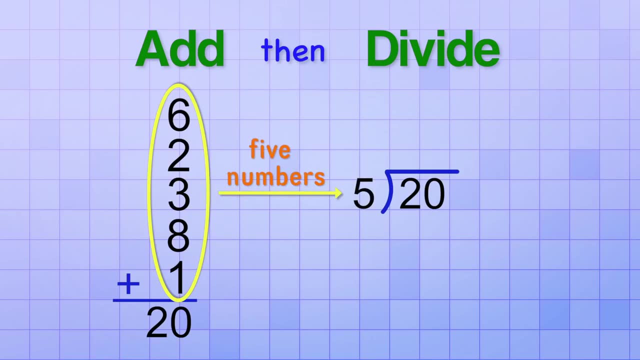 So that's the math procedure you use to find the mean of a dataset. It's just two simple steps. First you add up all the numbers in the set and then you divide the total you get by how many numbers you added up. 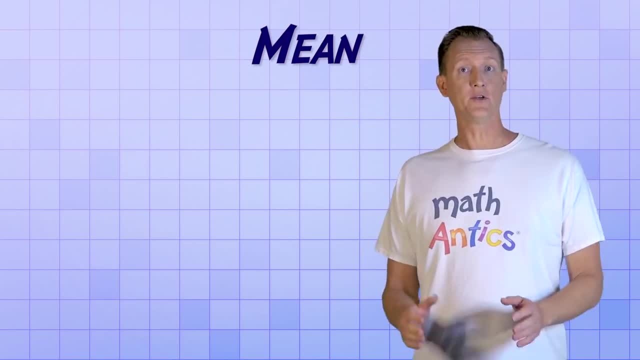 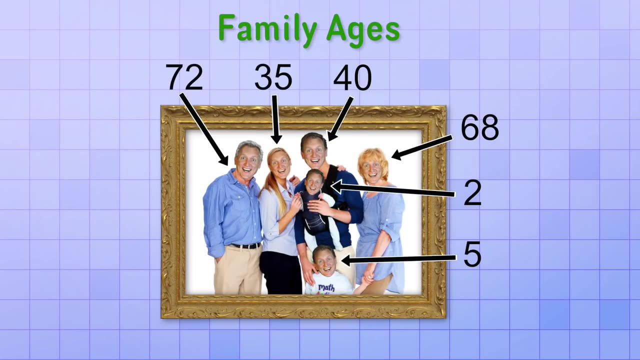 The answer you get is the mean of the dataset. Let's use that procedure to find the mean age of the members of this fine-looking group. If we add them all up using a calculator, or by hand if you'd like- the total of. 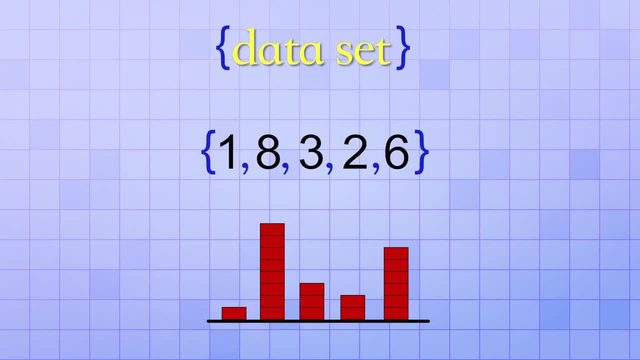 As a visual aid, let's also represent those numbers with stacks of blocks whose heights correspond to their values: 1, 8,, 3,, 2, 6.. Right now, since each of the five numbers is different, the stacks of blocks are all. 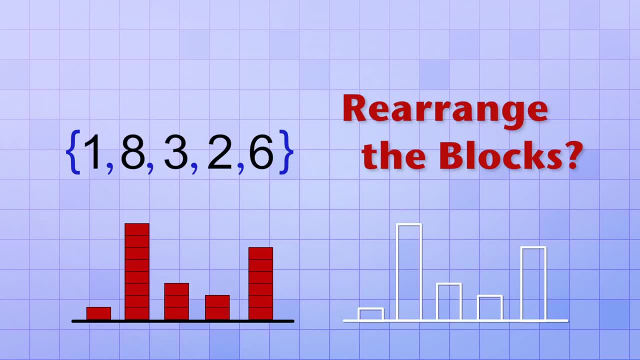 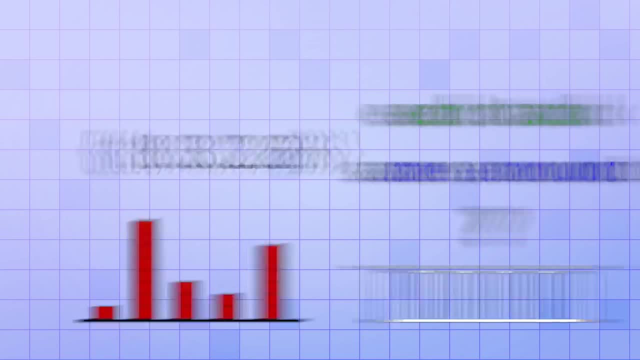 different heights. But what if we rearrange the blocks with the goal of making the stacks the same height? In other words, if each stack could have the exact same amount? what would that amount be? Well, with a bit of trial and error, you'll see that we have enough blocks for each stack. 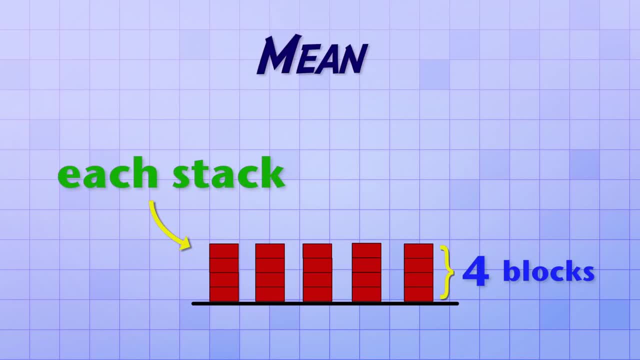 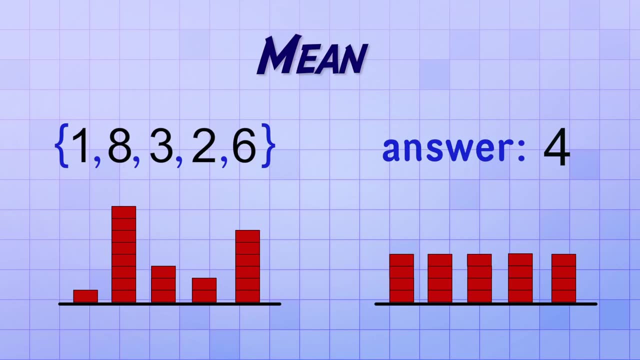 to have a total of 4.. That means that the mean or average for our original dataset would be 4.. Some of the numbers are greater than 4 and some are less, but if the amounts could all be made the same, they would all become 4.. 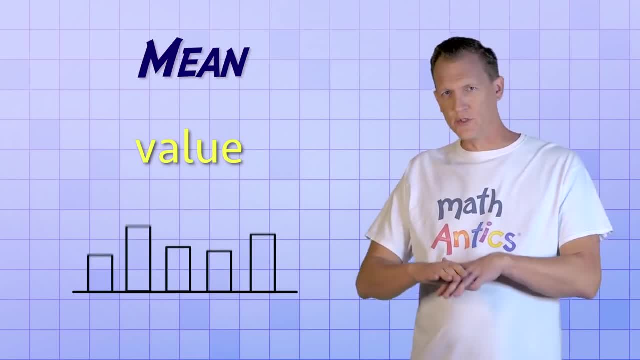 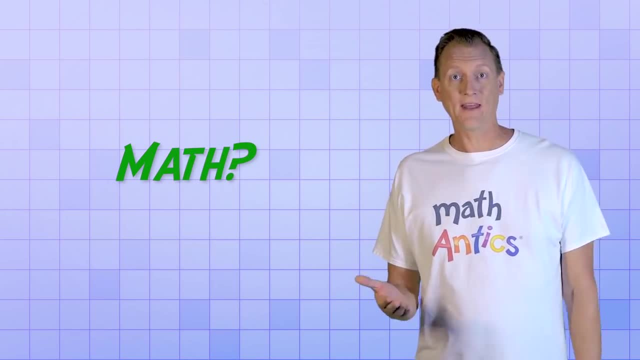 So that's the concept of the mean. It's the value you'd get if you could smooth out or flatten all of the different data values into one consistent value. But is there a way that we could use math to calculate the mean of a dataset? 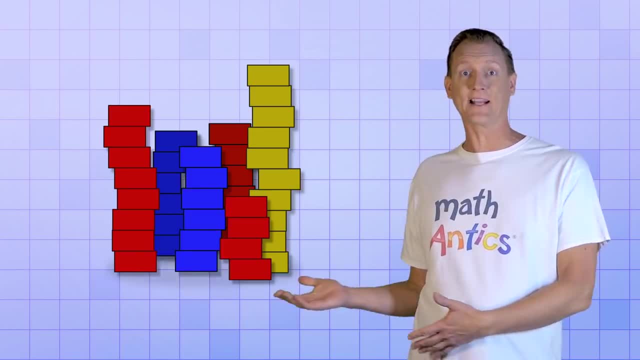 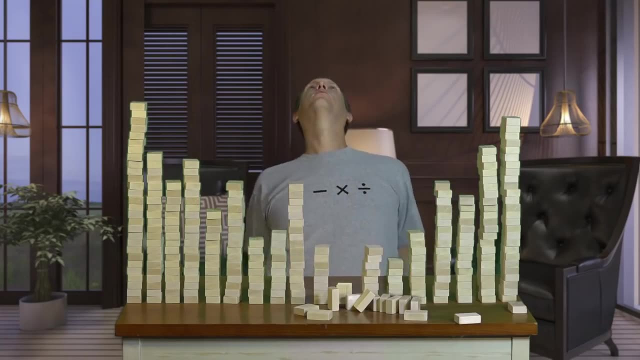 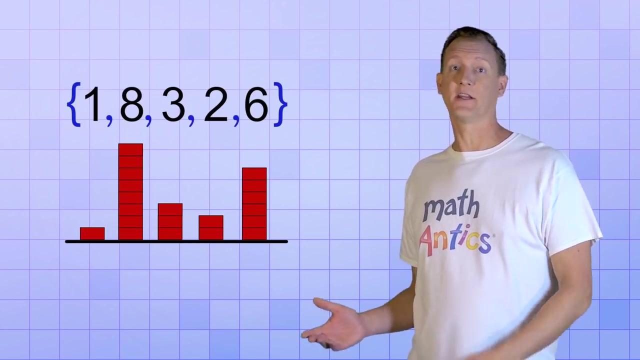 After all, it would be very inconvenient if we always had to use stacks of blocks to do it. There's gotta be an easier way. Oh man, Phew, It's easier for calculating the mean. let's start with blocks again, but this time instead. 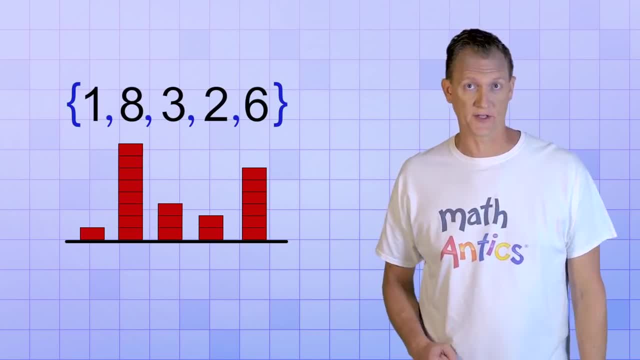 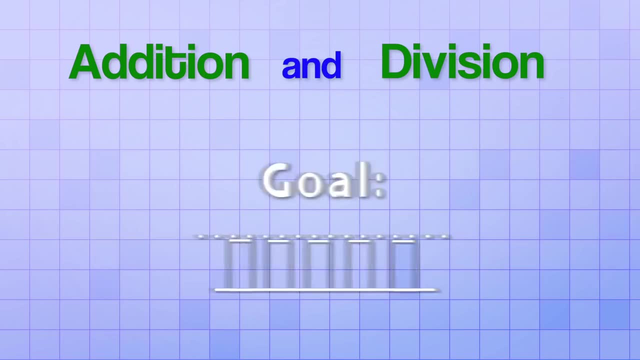 of using trial and error, let's use a more systematic way to make the stacks all the same height. This way involves a clever combination of addition and division. We know that we want to end up with 5 stacks that all have the same number of blocks, right? 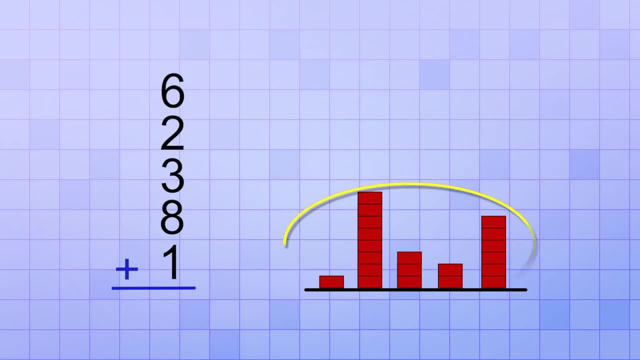 So first let's add up all of the numbers, which is like putting all of the blocks we have into one big stack. Adding up all of the numbers, or counting all the blocks, shows us that we have a total of 20.. 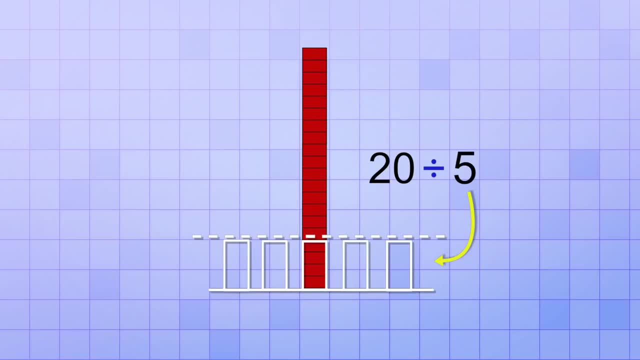 Next, Let's divide the total number, or stack, into 5 equal parts. Since the stack has a total of 20 blocks, dividing it into 5 equal stacks means that we'll have 4 in each, since 20 divided by 5 equals 4.. 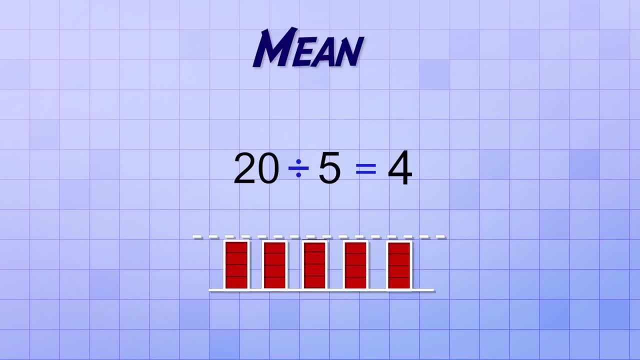 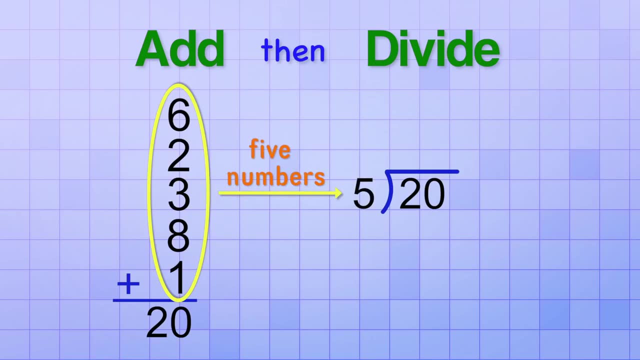 So that's the math procedure you use to find the mean of a dataset. It's just two simple steps. First you add up all the numbers in the set and then you divide the total you get by how many numbers you added up. 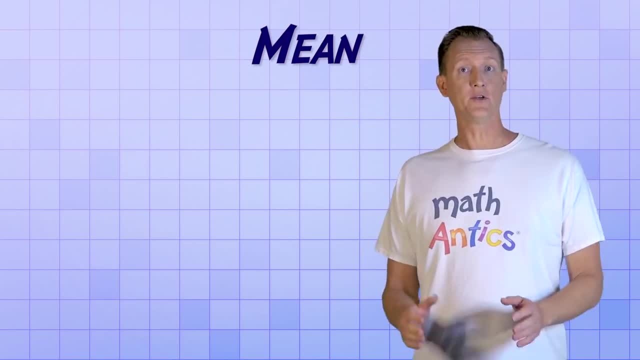 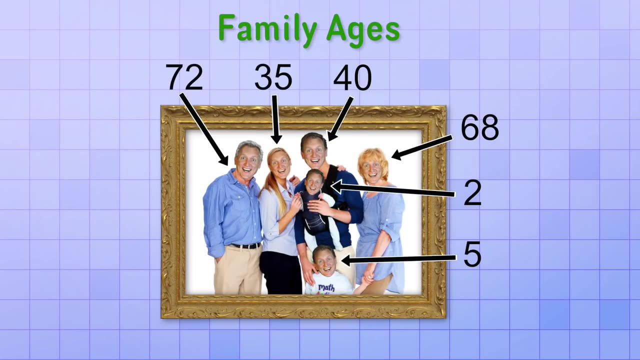 The answer you get is the mean of the dataset. Let's use that procedure to find the mean age of the members of this fine-looking group. If we add them all up using a calculator, or by hand if you'd like- the total of. 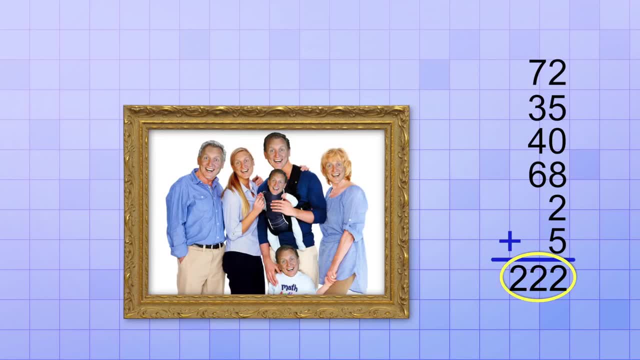 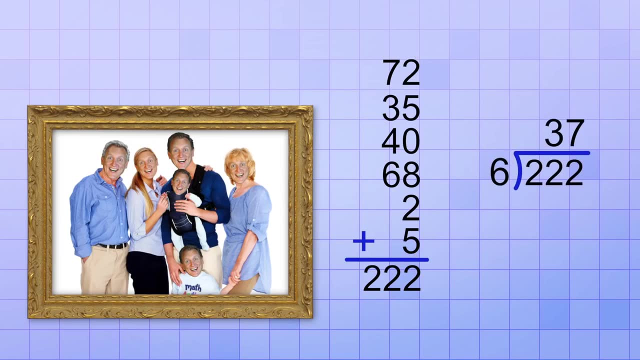 the ages is 222 years, But then we need to divide that total by the number of ages we added, which is 6.. 222 divided by 6 is 37.. So that's the mean age of all the members in this family. 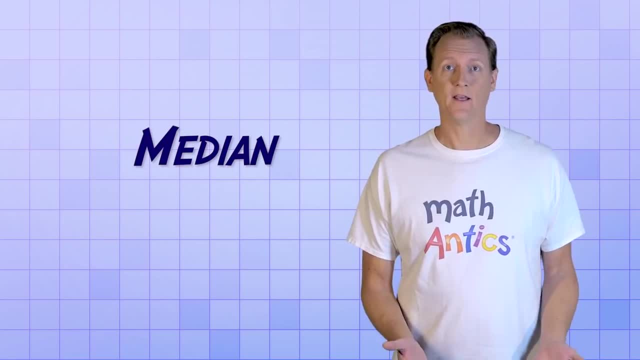 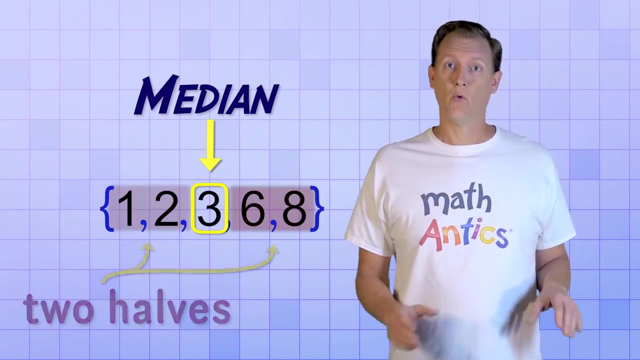 Alright, that's the mean. Now what about the median? The median is the middle of a dataset. It's the number that splits the dataset into two equally sized groups or halves. One half contains members that are greater than or equal to the median and the other 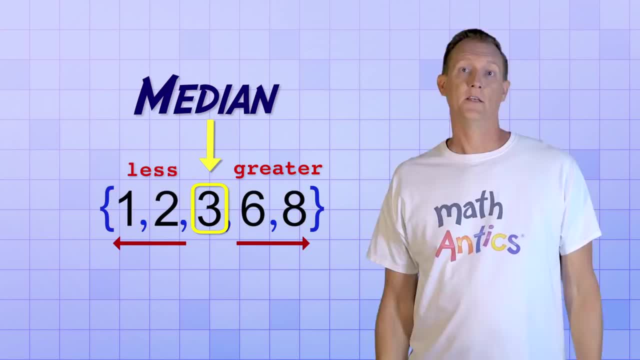 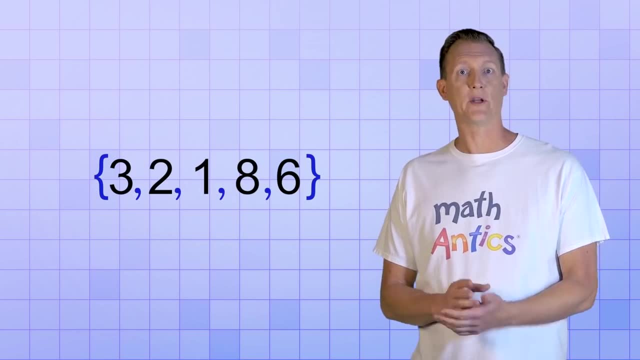 half contains members that are less than or equal to the median. Sometimes finding the median of a dataset is easy and sometimes it's hard. That's because finding the middle value of a dataset requires that its members be in order from the least to the greatest, or vice versa. 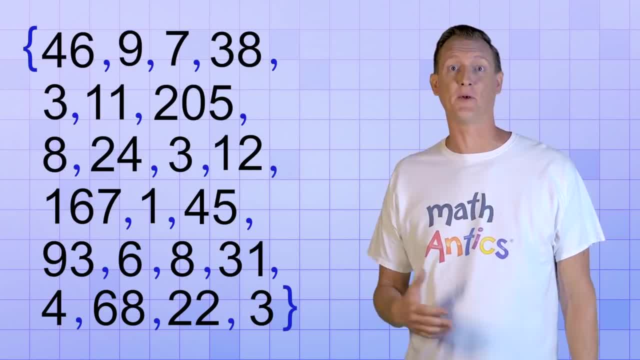 And if the dataset has a lot of numbers, it might take a lot of work to put them in the right order… if they aren't already that way. So to make things easier, let's start with a really basic dataset that isn't a whole. 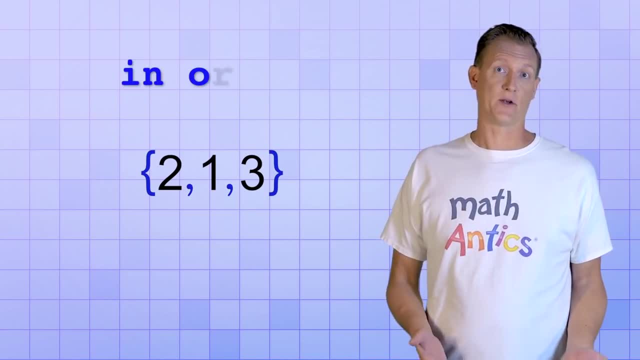 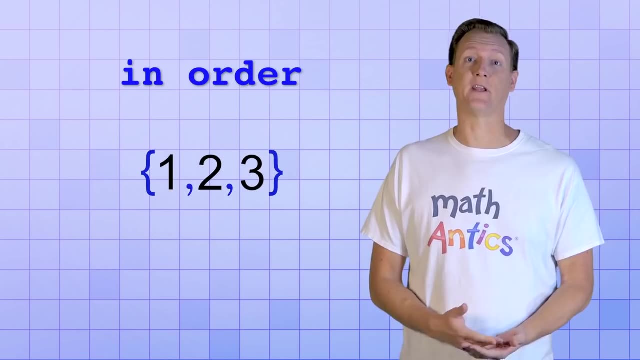 set of numbers. It's pretty easy to see that we can put this dataset in order from the least to the greatest value just by switching the 2 and the 1.. There now we have the dataset 1,, 2,, 3, and finding the median or middle of this dataset. 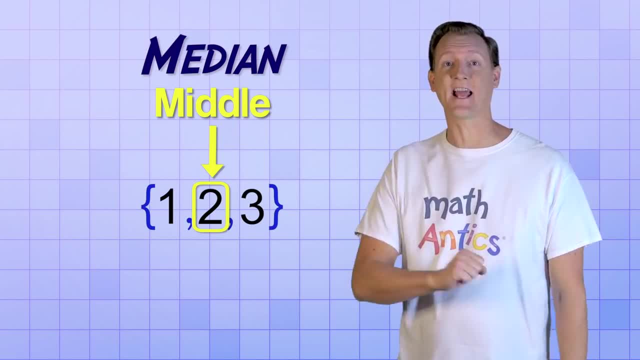 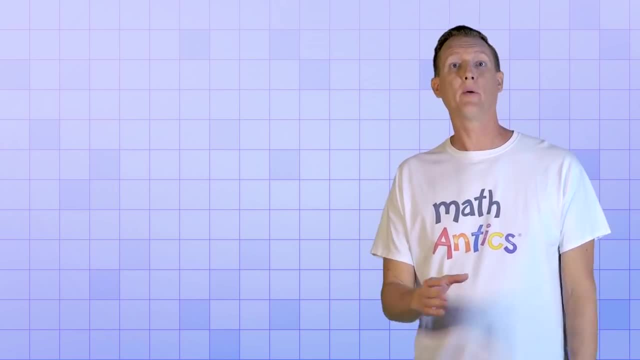 is easy, It's just 2, because the 2 is located exactly in the middle. That almost seems too easy, doesn't it? But don't worry, it gets harder. But before we try a harder problem, I want to point out that sometimes the mean and the 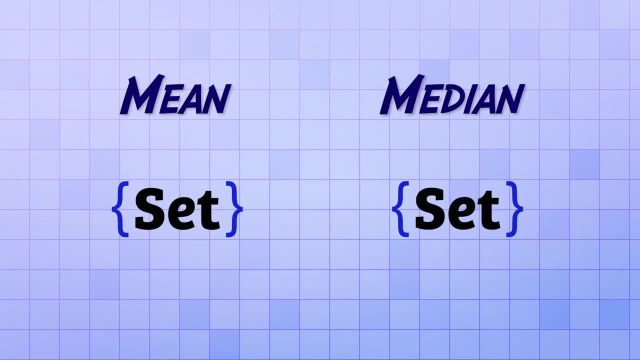 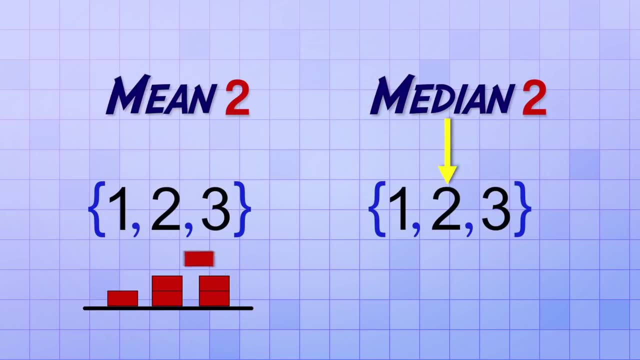 median of a dataset are the same number and sometimes they're not. In the case of our simple dataset, 1,, 2,, 3,, the median is 2, and the mean is also 2,. as you can see, if we rearrange the amounts or follow the procedure we learned to calculate. 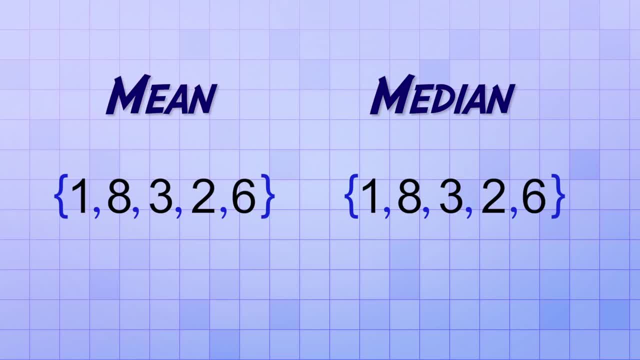 the mean. But what about the first dataset that we found the mean of? We determined that the mean of this dataset is 4, but what about the median? Well, the median is the middle and since this dataset is already in order from least, 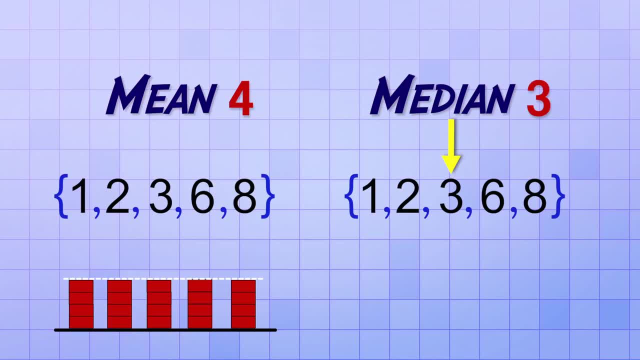 to greatest. it's easy to see that the 3 is located in the middle, since it splits the other members into two equal groups. So for this dataset the mean is 4, but the median is 3.. So to find the median of a set of numbers, first you need to make sure that all the numbers 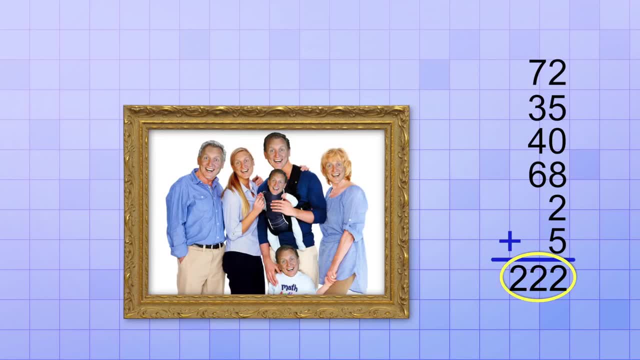 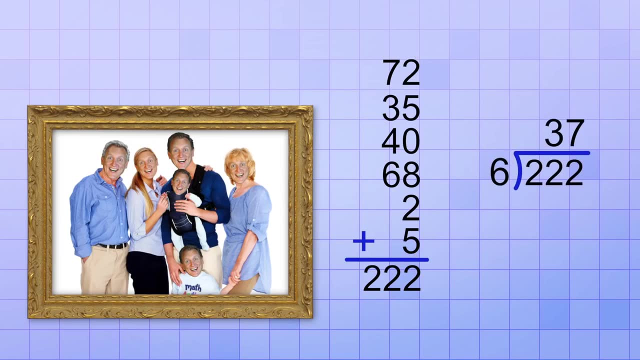 the ages is 222 years, But then we need to divide that total by the number of ages we added, which is 6.. 222 divided by 6 is 37.. So that's the mean age of all the members in this family. 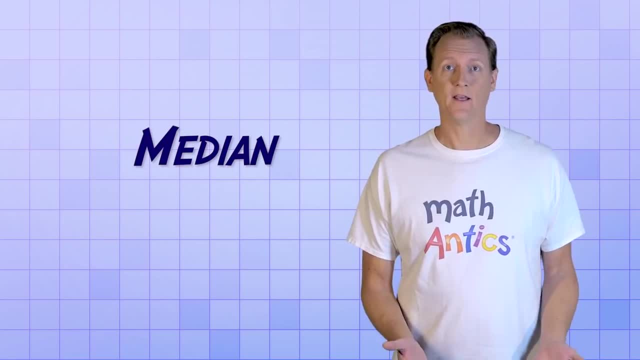 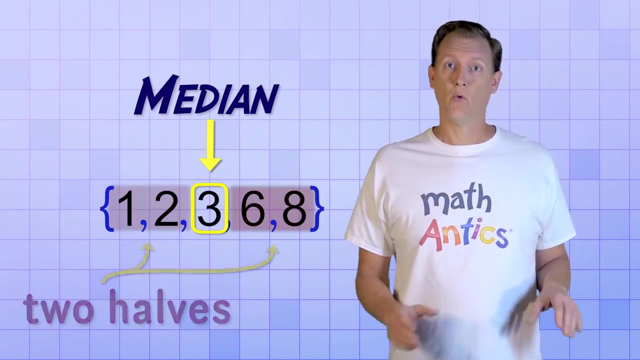 Alright, that's the mean. Now what about the median? The median is the middle of a dataset. It's the number that splits the dataset into two equally sized groups or halves. One half contains members that are greater than or equal to the median and the other 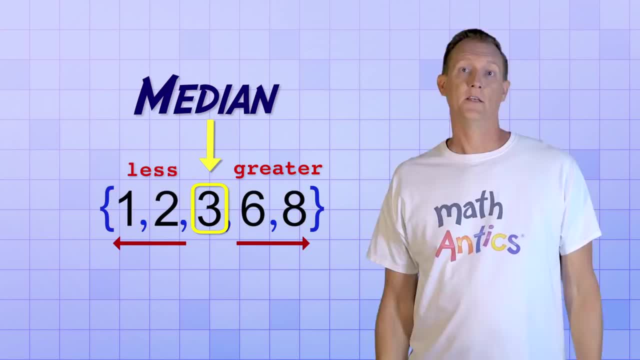 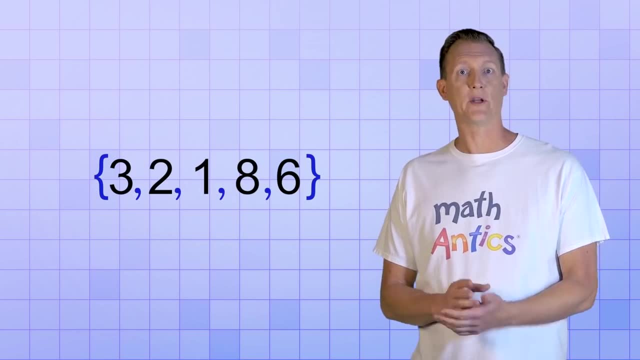 half contains members that are less than or equal to the median. Sometimes finding the median of a dataset is easy and sometimes it's hard. That's because finding the middle value of a dataset requires that its members be in order from the least to the greatest, or vice versa. 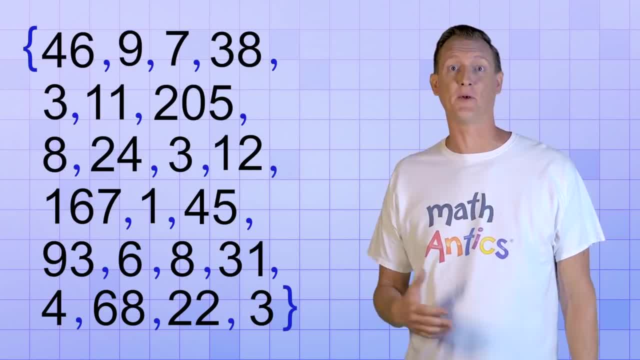 And if the dataset has a lot of numbers, it might take a lot of work to put them in the right order… if they aren't already that way. So to make things easier, let's start with a really basic dataset that isn't a whole. 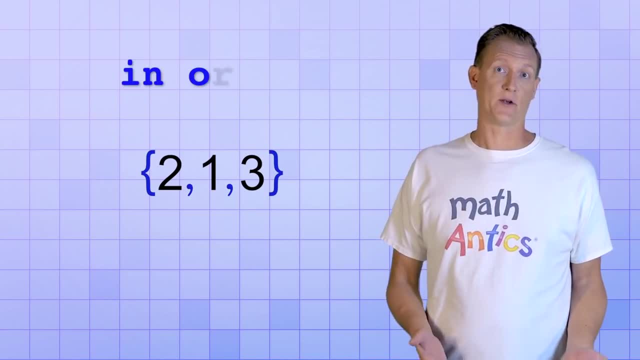 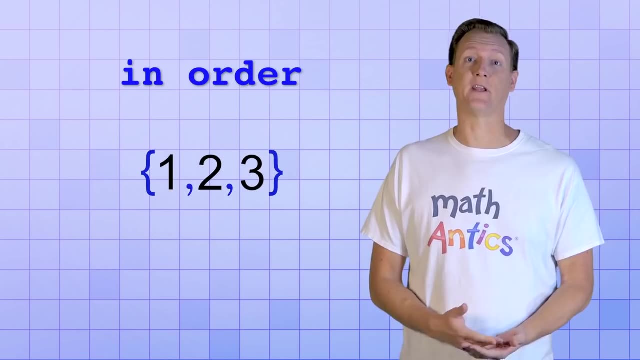 set of numbers. It's pretty easy to see that we can put this dataset in order from the least to the greatest value just by switching the 2 and the 1.. There now we have the dataset 1,, 2,, 3, and finding the median or middle of this dataset. 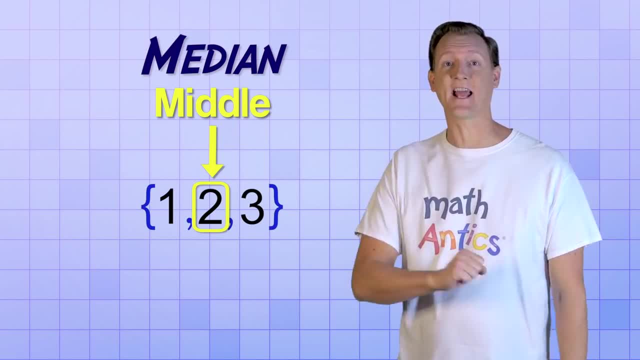 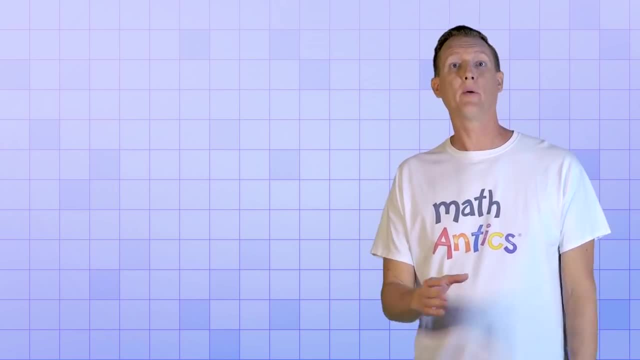 is easy, It's just 2, because the 2 is located exactly in the middle. That almost seems too easy, doesn't it? But don't worry, it gets harder. But before we try a harder problem, I want to point out that sometimes the mean and the 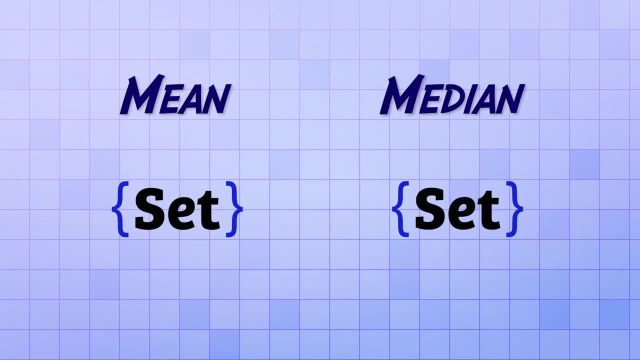 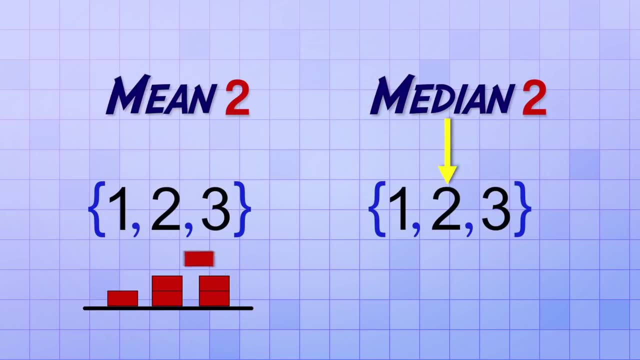 median of a dataset are the same number and sometimes they're not. In the case of our simple dataset, 1,, 2,, 3,, the median is 2, and the mean is also 2,. as you can see, if we rearrange the amounts or follow the procedure we learned to calculate. 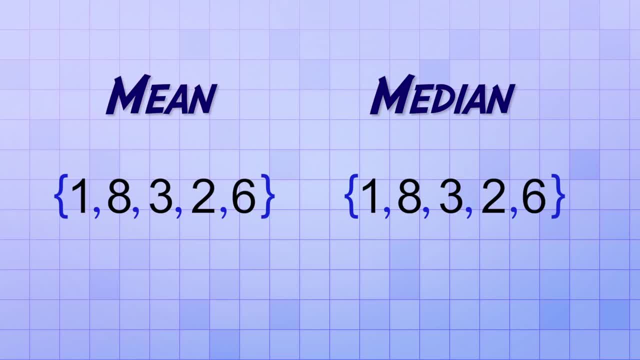 the mean. But what about the first dataset that we found the mean of? We determined that the mean of this dataset is 4, but what about the median? Well, the median is the middle and since this dataset is already in order from least, 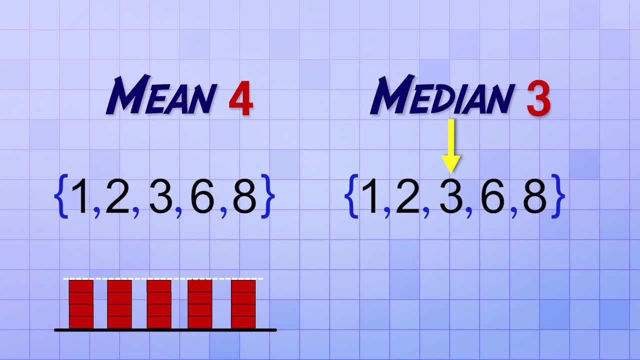 to greatest. it's easy to see that the 3 is located in the middle, since it splits the other members into two equal groups. So for this dataset the mean is 4, but the median is 3.. So to find the median of a set of numbers, first you need to make sure that all the numbers 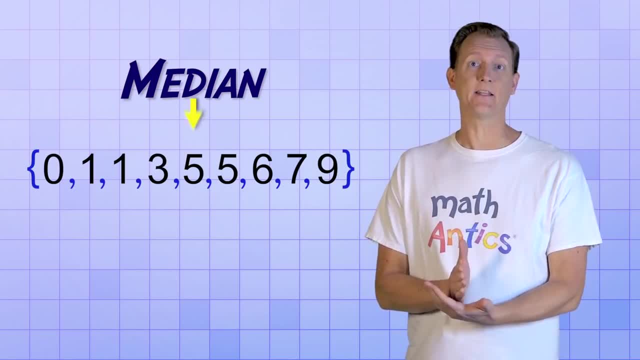 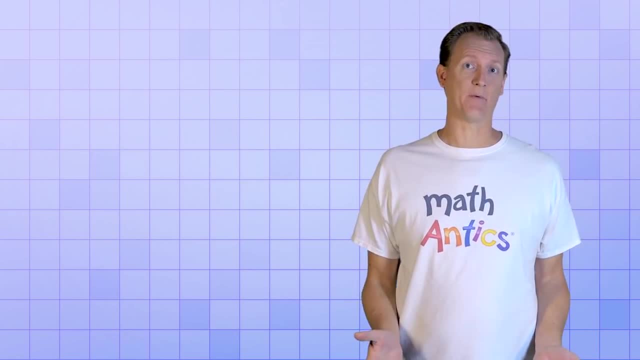 are in order, and then you can identify the member that's exactly in the middle by making sure there's an equal number of members on either side of it. Okay, so far, so good. But some of you may be wondering what if a dataset doesn't have an obvious middle member? 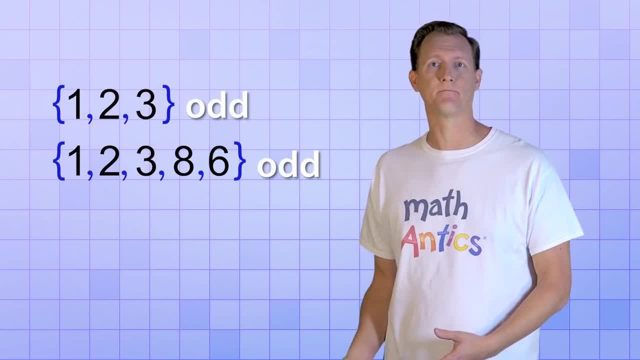 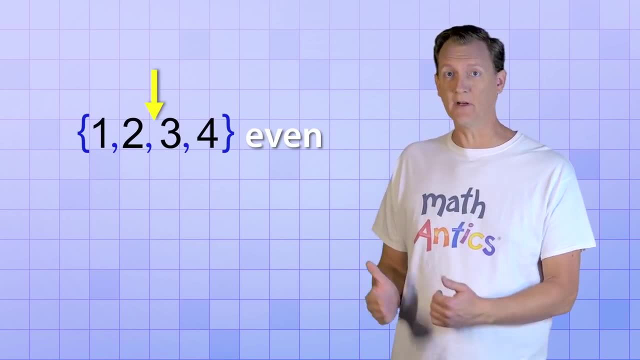 All of the sets we've found the median of so far- have an odd number of members. But what if a set has an even number of members, Like this one, Like the dataset 1,, 2,, 3,, 4? There isn't a member in the middle that splits the set into two equally sized groups. 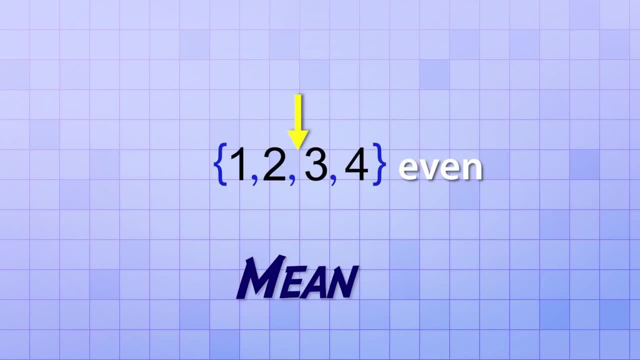 If that's the case, we can actually use what we learned about the mean to help us out. If the dataset has an even number of members, then to find the median we need to take the middle two numbers and calculate the mean or average of those two. 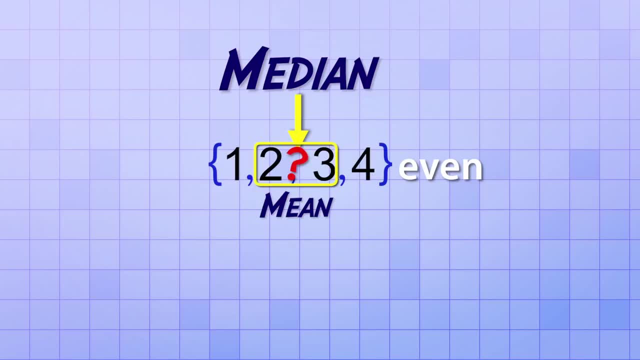 By doing that, we're basically figuring out what number would be exactly halfway between the two middle numbers, and that number will be our median In the set 1, 2, 3, 4,. we need to take the middle two numbers- 2 and 3, and find the. 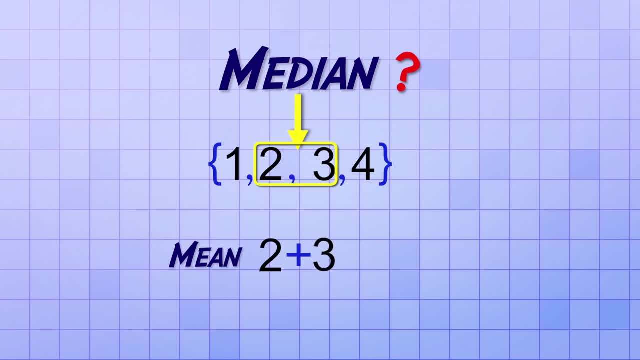 mean of those numbers. We can do that by adding 2 and 3, and then dividing by 2.. 2 plus 3 equals 5, and 5 divided by 2 is 2.5. So the median of the dataset is 2.5. 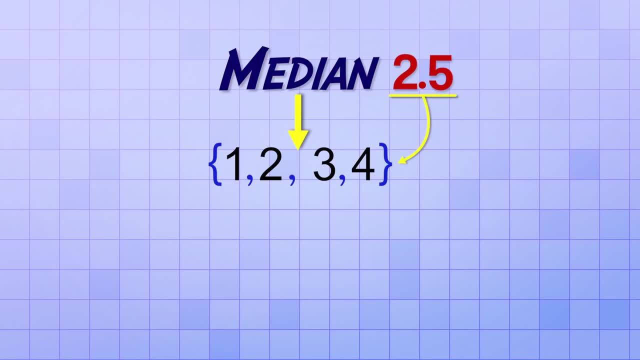 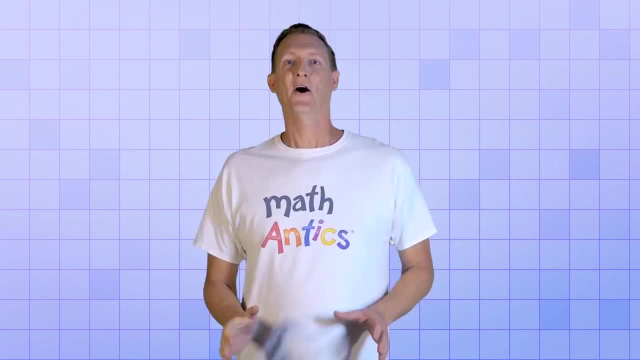 Even though the number 2.5 isn't actually a member of the dataset, it's the median, because it represents the middle of the dataset and it splits the members into two equally sized groups. Okay, So now you know the difference between mean and median, but what about the MODE of a dataset? 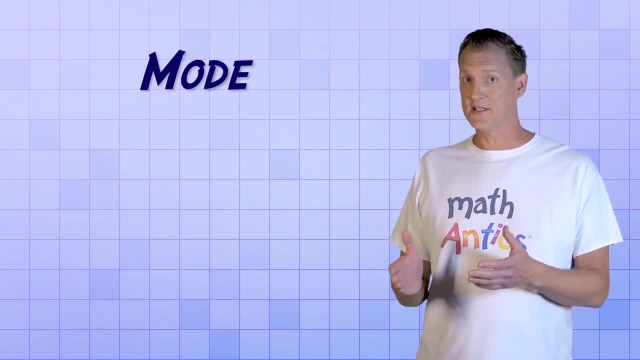 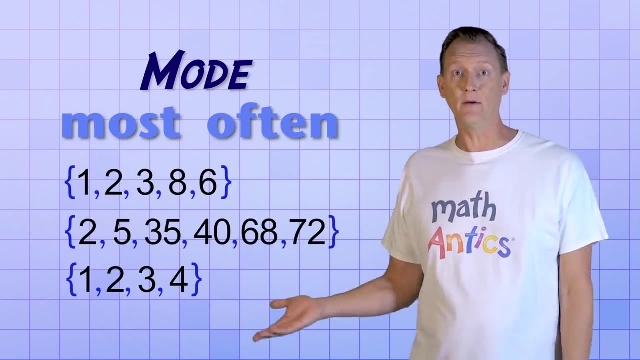 What in the world does that mean? Well, mode is just a technical word for the value in a dataset that occurs most often In the datasets we've seen so far, there hasn't even been a mode, because none of the data values were ever repeated. 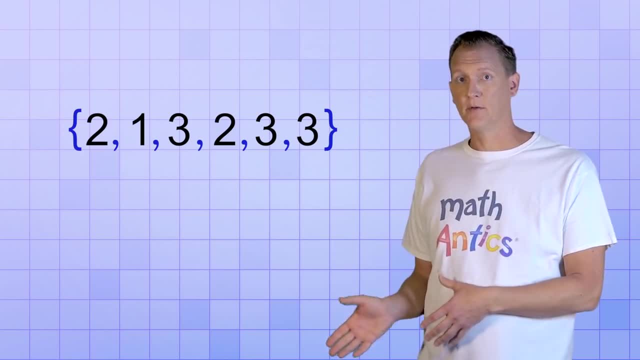 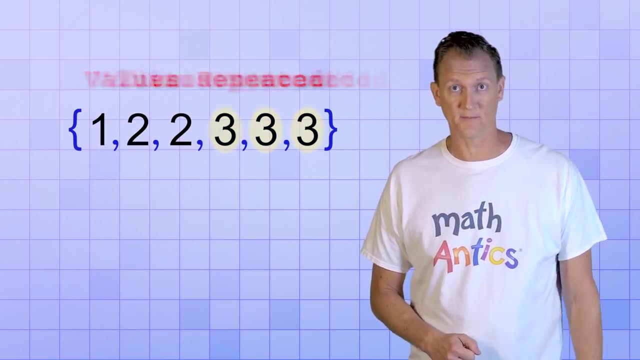 But what if you had this dataset? This set has six members, but some of the values are repeated. If we rearrange them, you can see that there's one 1, two 2s and three 3s. The mode of this dataset is the value that occurs most often or most frequently, so 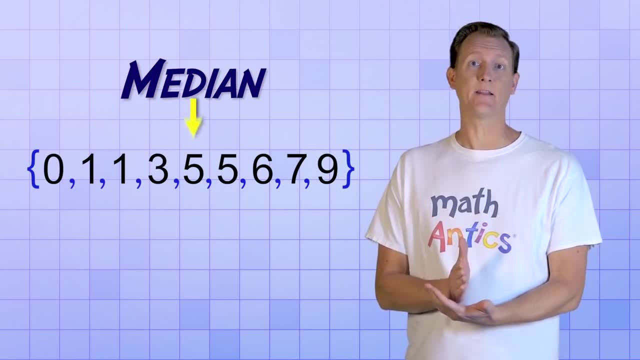 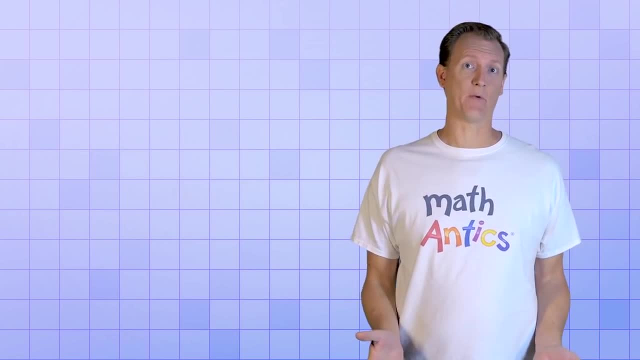 are in order, and then you can identify the member that's exactly in the middle by making sure there's an equal number of members on either side of it. Okay, so far, so good. But some of you may be wondering what if a dataset doesn't have an obvious middle? 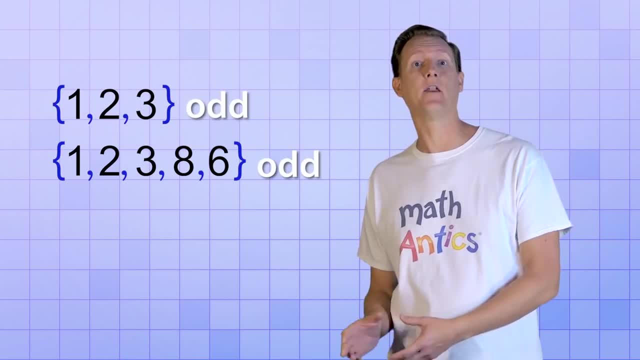 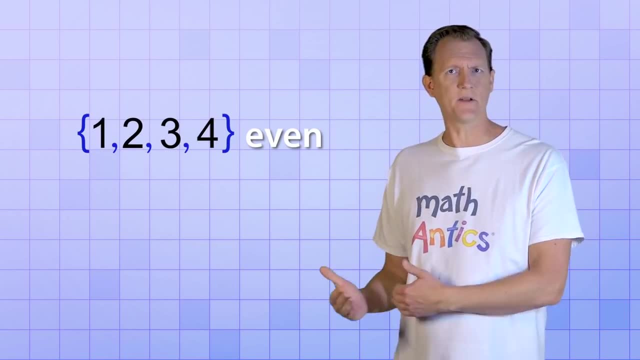 member. All of the sets we've found the median of so far have an odd number of members. But what if a set has an even number of members, Like the dataset 1,, 2,, 3,, 4? There isn't a member in the middle that splits the set into two equally sized groups. 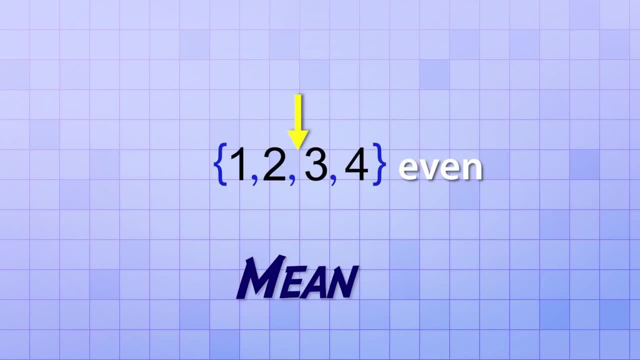 If that's the case, we can actually use what we learned about the mean to help us out. If the dataset has an even number of members, then to find the median we need to take the middle two numbers and calculate the mean or average of those two. 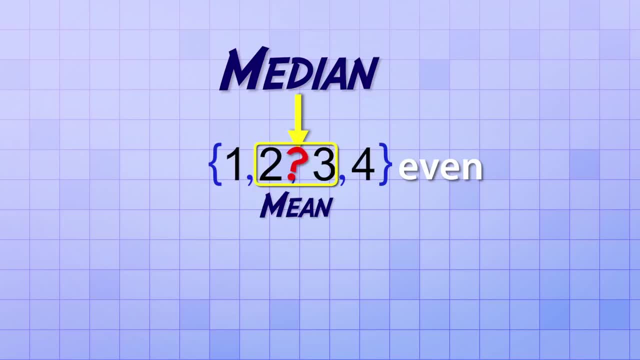 By doing that, we're basically figuring out what number would be exactly halfway between the two middle numbers, and that number will be our median. For example, in the set 1, 2, 3, 4,, we need to take the middle two numbers, 2 and 3, and 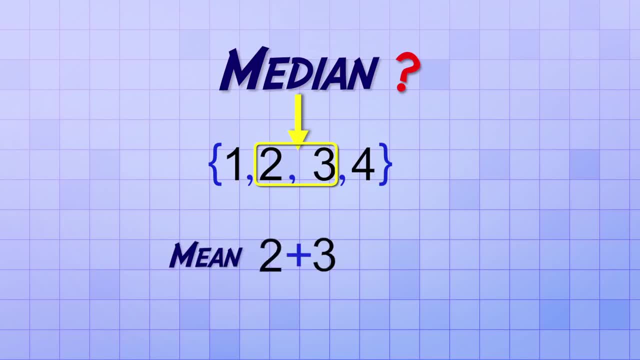 find the mean of those numbers. We can do that by adding 2 and 3, and then dividing by 2.. 2 plus 3 equals 5, and 5 divided by 2 is 2.5. So the median of the dataset is 2.5. 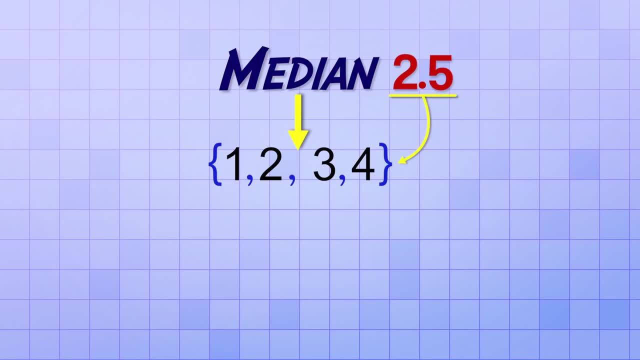 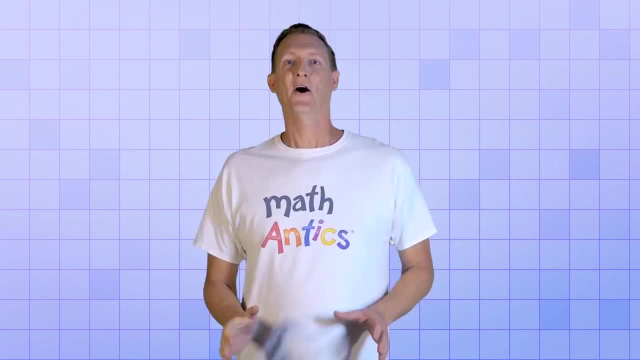 Even though the number 2.5 isn't actually a member of the dataset, it's the median because it represents the middle of the dataset and it splits the members into two equally sized groups. Okay, So now you know the difference between mean and median, but what about the mode of a dataset? 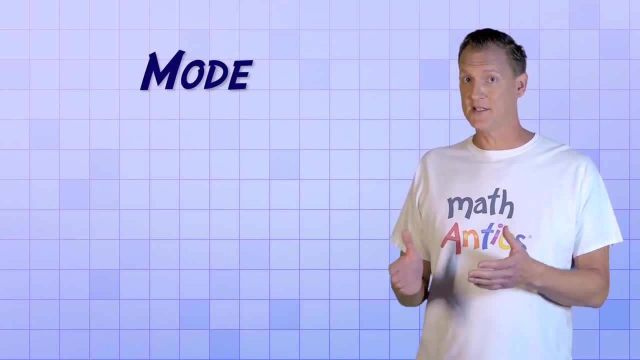 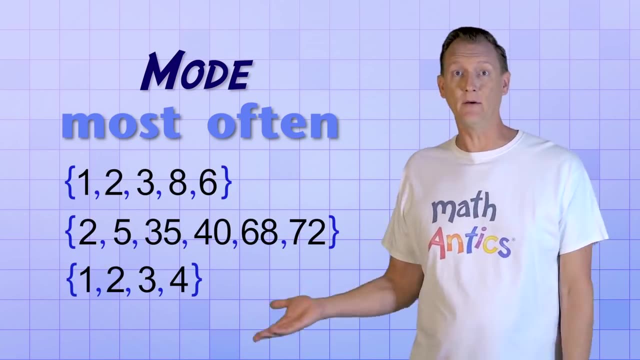 What in the world does that mean? Well, mode is just a technical word for the value in a dataset that occurs most often In the datasets we've seen so far, there hasn't even been a mode, because none of the data values were ever repeated. 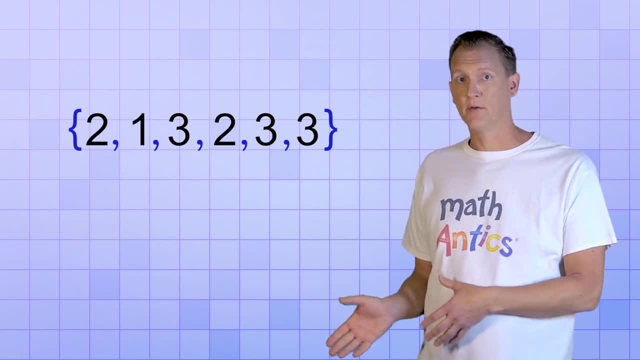 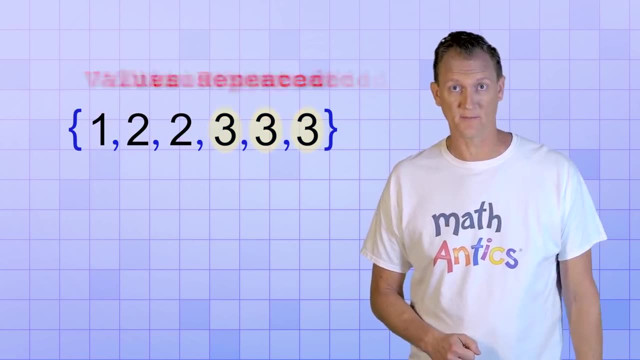 But what if you had this dataset? This set has six members, but some of the values are repeated. If we rearrange them, you can see that there's one 1, two 2s and three 3s. The mode of this dataset is the value that occurs most often or most frequently, so 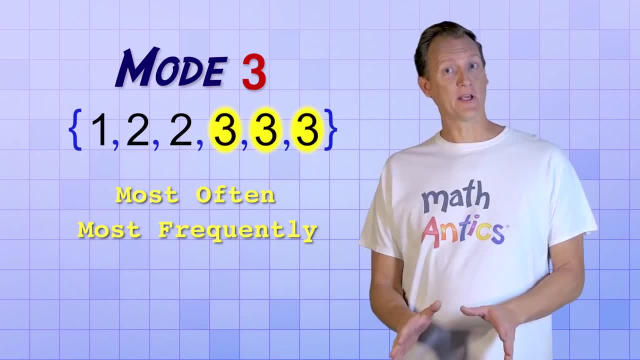 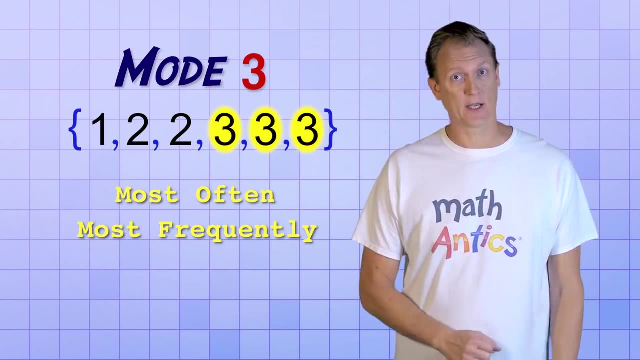 that would be 3, since there's three 3s Now don't get confused just because the number 3 was repeated three times. The mode is the number that's repeated most often, not how many times it was repeated. As I mentioned, if each member in a dataset occurs only once, it has no mode. 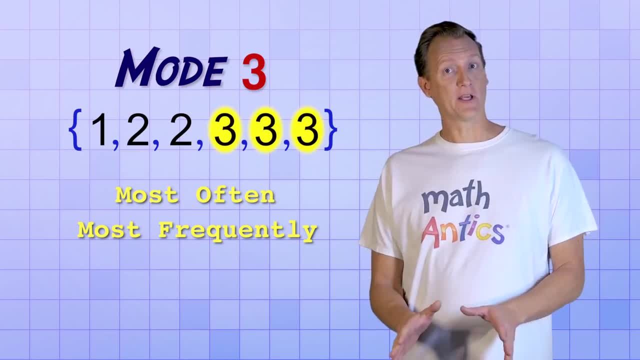 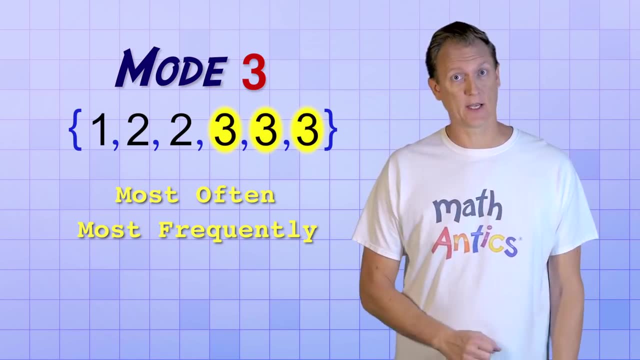 that would be 3, since there's three 3s Now don't get confused just because the number 3 was repeated three times. The mode is the number that's repeated most often, not how many times it was repeated. As I mentioned, if each member in a dataset occurs only once, it has no mode. 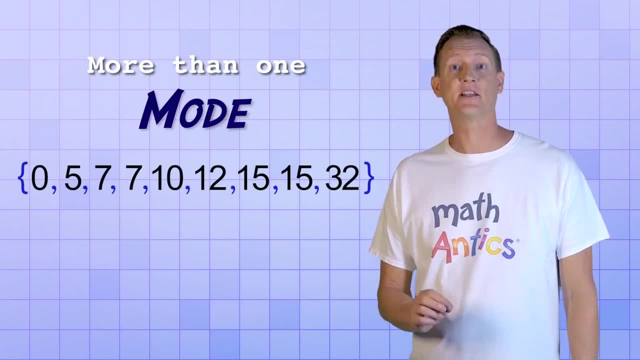 But it's also possible for a dataset to have more than one mode. Here's an example of a dataset like that. In this set, the number 7 is repeated twice, but the number 7 is repeated twice, so it's the number 15.. 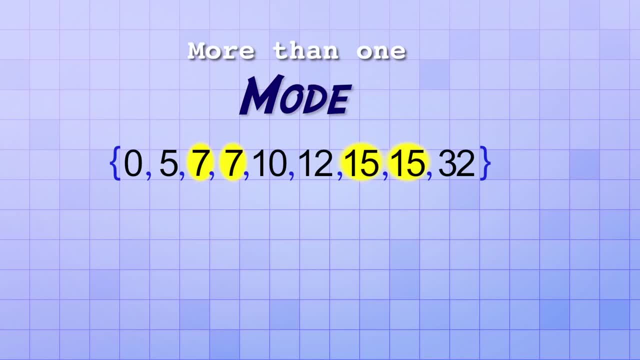 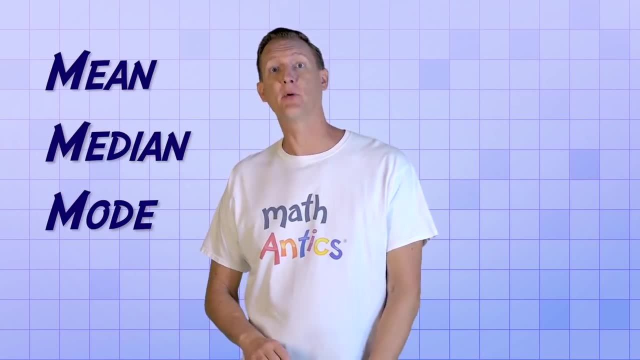 That means they tie for the title of the mode. This set has two modes, 7 and 15.. OK, so now that you know what the mean median and mode of a dataset are, let's put all that new information to use in one final real-world example. 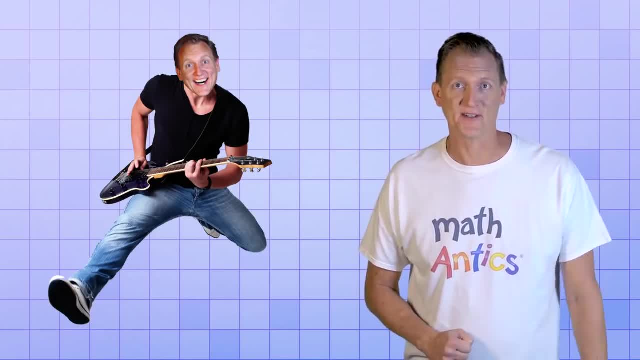 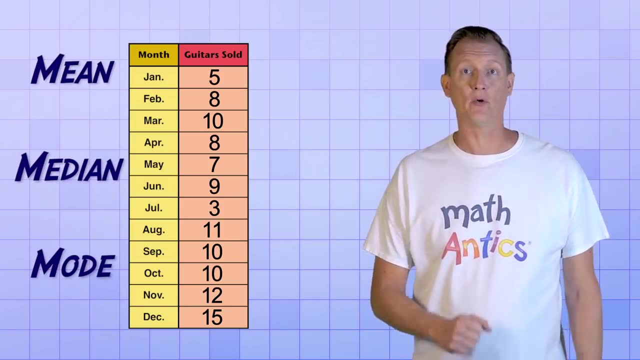 Suppose there's this guy who makes and sells custom electric guitars. Here's a table showing how many guitars he sold during each month of the year. Let's find the mean, median and mode of this dataset. 1. To find the mean, we need to add up the number of guitars sold in each month. 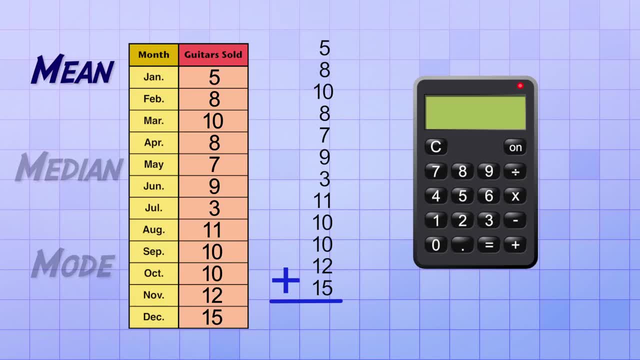 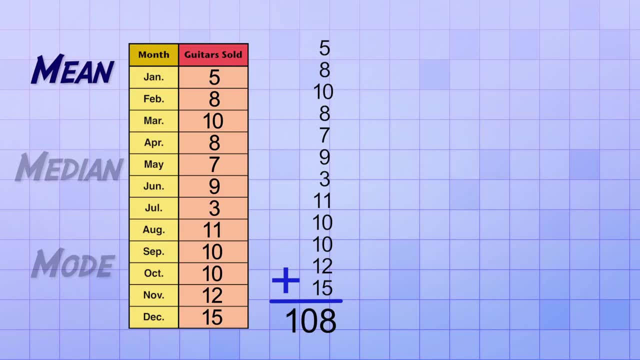 You can do the addition by hand or you can use a calculator if you want to Either way. be careful, since that's a lot of numbers to add up and we don't want to make a mistake. The answer I get is 108.. 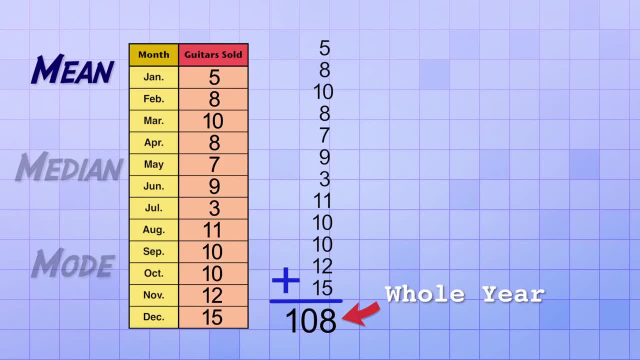 So that's the total he sold for the whole year. But to get the mean sold each month we need to divide that total by the number of months, which is 12.. 108 divided by 12 is 9.. So the mean, or average, is 9.. 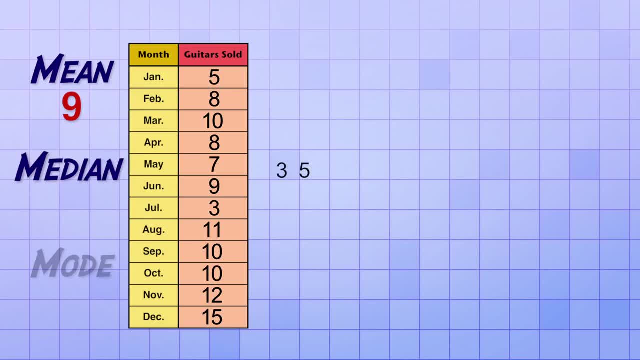 2. To find the median of the dataset, we're going to have to rearrange the 12 data points in order from smallest to largest, so we can figure out what the middle value is There. That's better, Since there's an even number of members in this set, we can't just choose the middle. 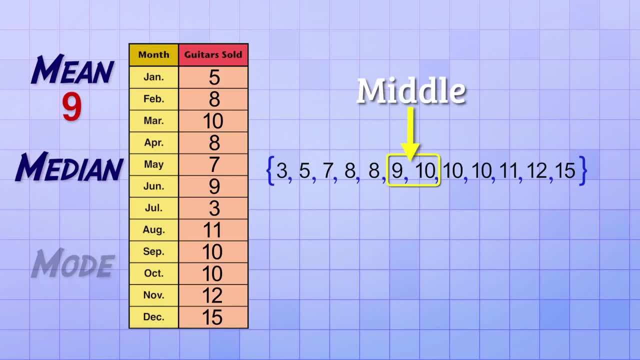 number. So we're going to have to pick the middle two numbers and then find the mean of them. 9 and 10 are in the middle, since there's an equal number of data values on either side of them, So we need to take the mean of 9 and 10.. 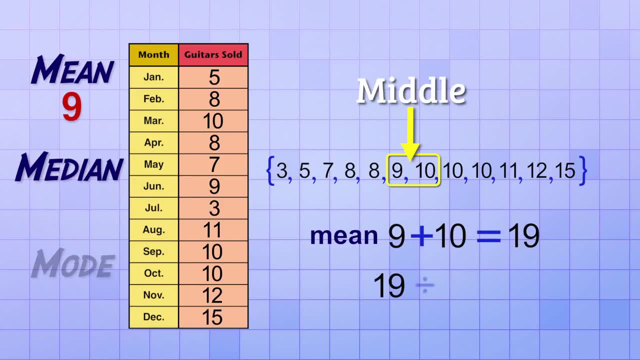 That's easy: 9 plus 10 equals 19.. And then 19 divided by 2 is 9.5.. So we need to take the mean of 9 and 10.. That's 9.5.. So the median number of guitars sold is 9.5.. 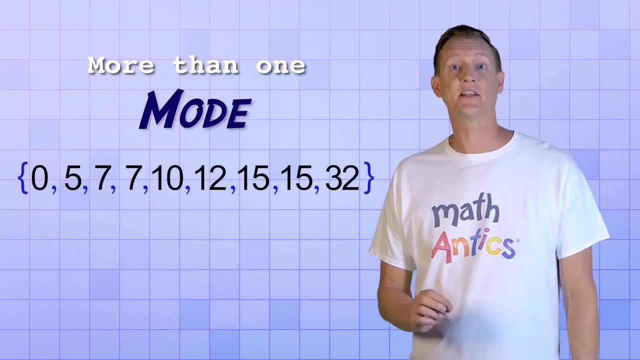 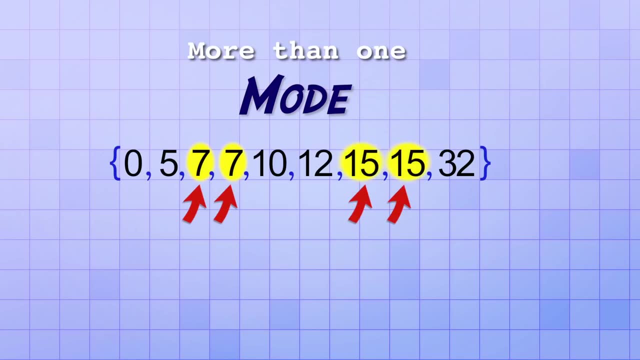 But it's also possible for a dataset to have more than one mode. Here's an example of a dataset like that. In this set the number 7 is repeated twice, But so is the number 15. That means they tie for the title of the mode. 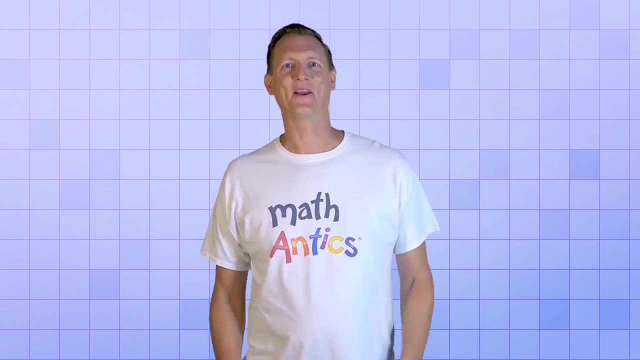 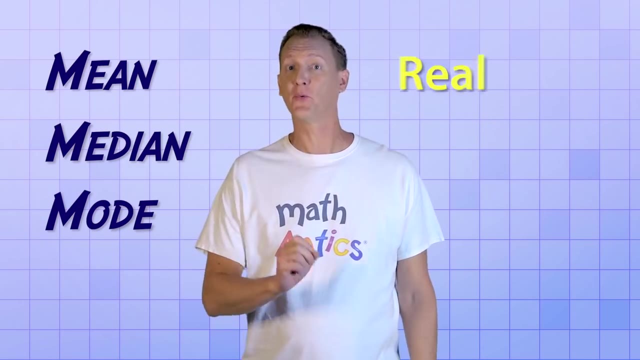 This set has two modes, 7 and 15.. Okay, so now that you know what the mean median and mode of a dataset are, let's put all that new information to use in one final real-world example. Suppose there's this guy who makes and sells custom electric guitars. 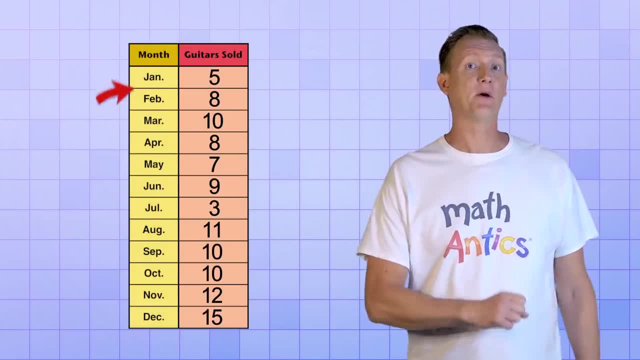 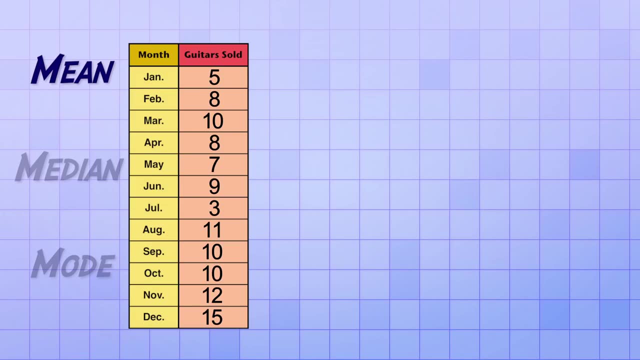 Here's a table showing how many guitars he sold during each month of the year. Let's find the mean, median and mode of this dataset First. to find the mean, we need to add up the number of guitars sold in each month. 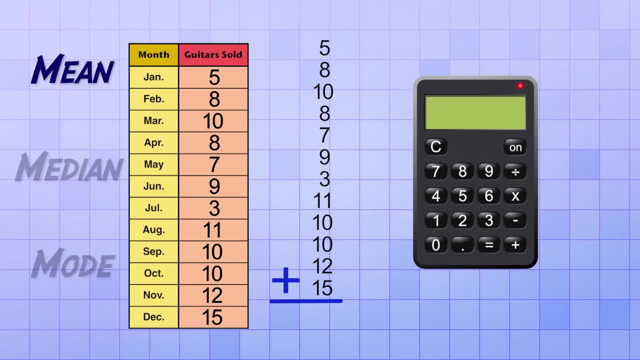 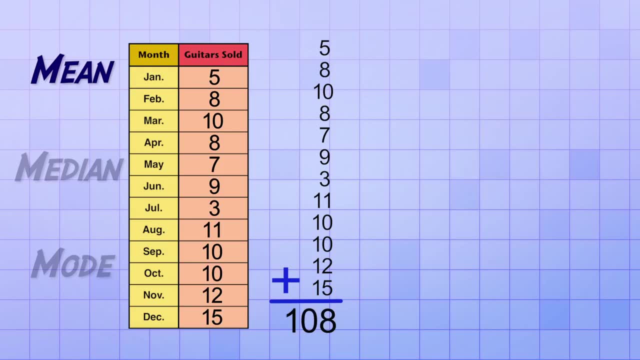 You can do the addition by hand or you can use a calculator if you want to Either way. be careful, since that's a lot of numbers to add up and we don't want to make a mistake. The answer I get is 108.. 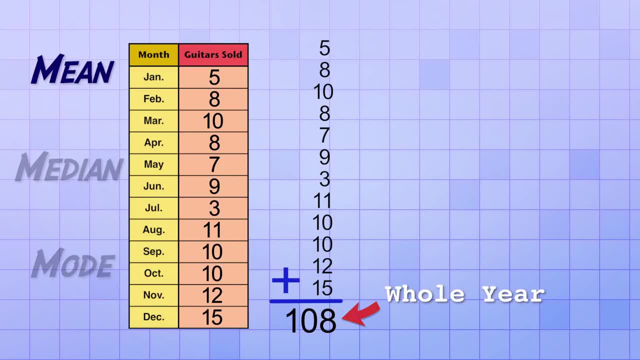 So that's the total he sold for the whole year. But to get the mean sold each month we need to divide that total by the number of months, which is 12.. 108 divided by 12 is 9.. So the mean, or average, is 9.. 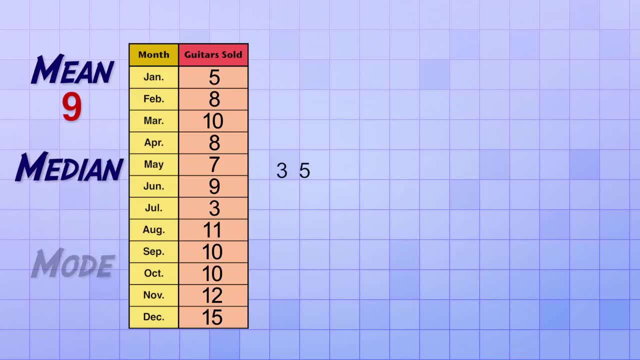 Next, to find the mean, median and mode of this dataset, we need to add up the number of guitars sold in each month. To find the median of the dataset, we're going to have to rearrange the 12 data points in order from smallest to largest. 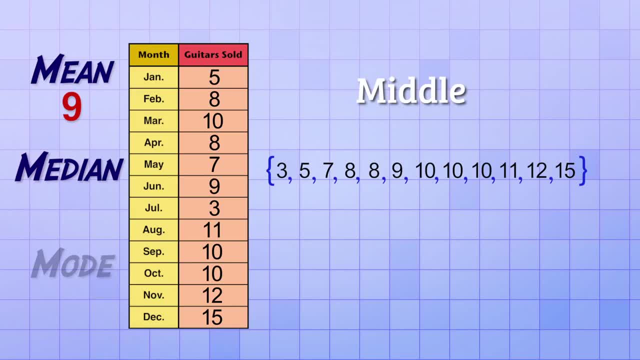 so we can figure out what the middle value is There. that's better, Since there's an even number of members in this set, we can't just choose the middle number, So we're going to have to pick the middle two numbers and then find the mean of them. 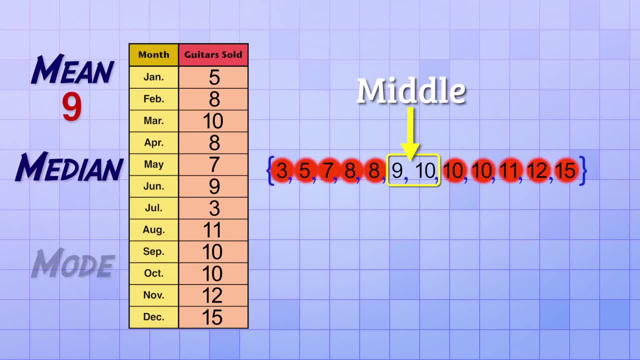 9 and 10 are in the middle, since there's an equal number of data values on either side of them, So we need to take the mean of 9 and 10.. That's easy. 9 plus 10 equals 19.. 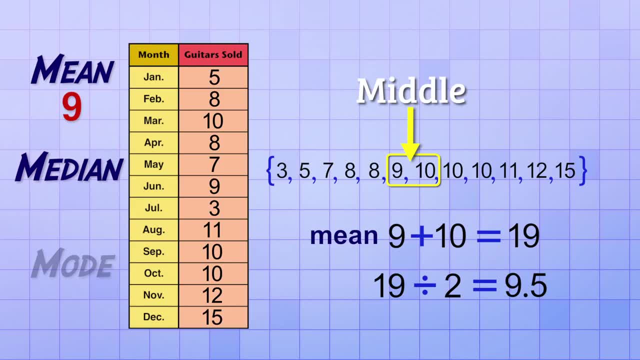 And then 19 divided by 2 is 9.2.. So the median number of guitars sold is 9.5.. That means that in half of the months he sold more than 9.5, and in half of the months he sold less than 9.5.. 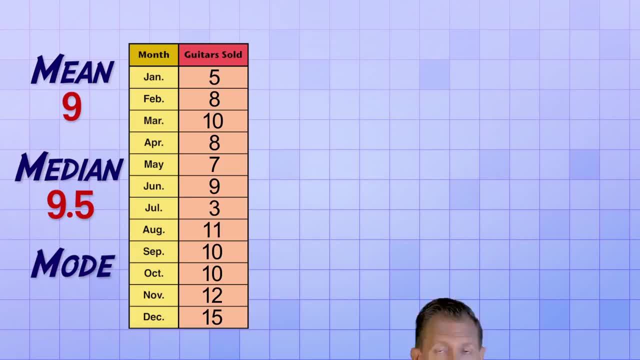 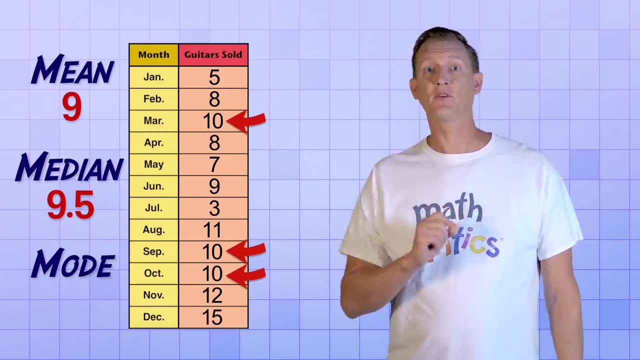 Last of all, let's identify the mode of this dataset. if there is one, Well, let's see. There's two 8s in the dataset, Oh, but there's three- 10s. That looks like the most frequent number.